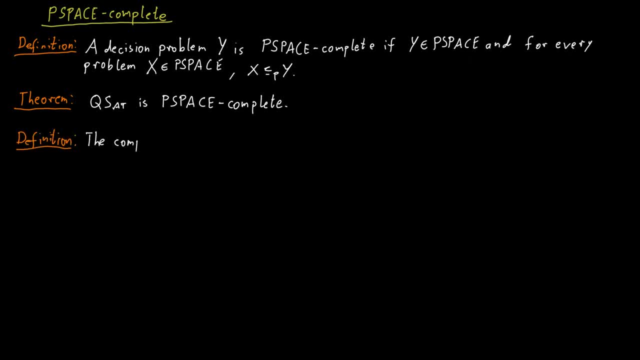 are solvable in polynomial time. The complexity class EXPTIME contains all the decision problems which are solvable in exponential time, which means there exists a Turing machine that solves those problems and its running time is bounded by an exponential function in the size of the input. So say, the size of the input is n and the 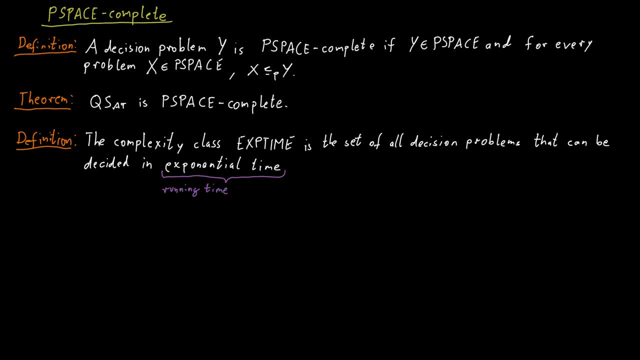 turing time is n, Then we allow a running time of the form 2 to the power of some polynomial function in n. The complexity class PSPACE is contained in the complexity class EXPTIME. We can prove this in several ways. One way is to use 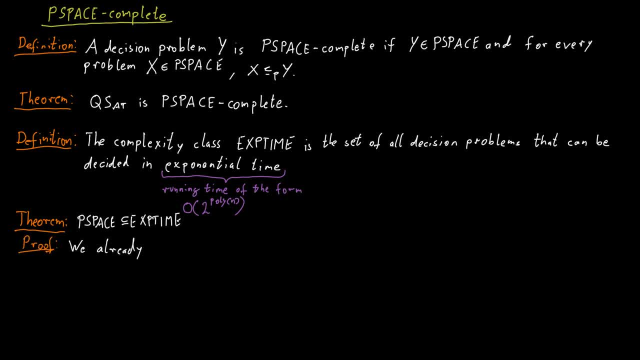 quantified satisfiability. Our previous algorithm already solves quantified satisfiability in exponential time. Now, since we know that quantified satisfiability is also PSPACE-complete, it means that we can solve all problems in PSPACE in exponential time, because we can simply reduce. 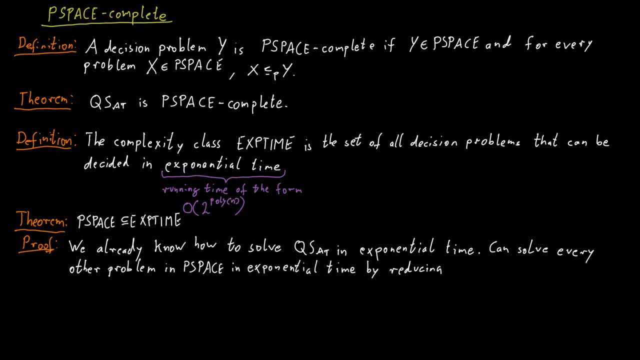 those problems to quantified satisfiability in polynomial time and then solve quantified satisfiability in exponential time. to get the answer to the original question, A different way of seeing that PSPACE is quantified satisfiability is to see a is contained in exp. time is maybe even nicer. 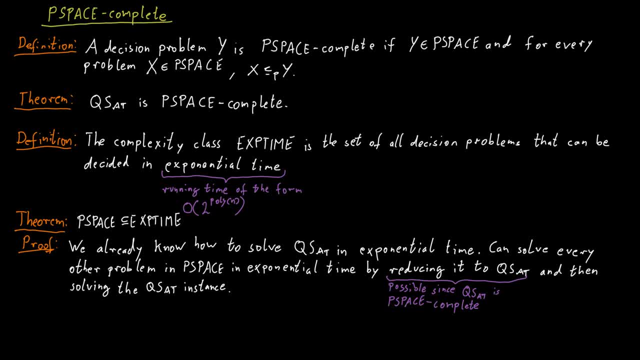 It doesn't use any advanced theorems like qsat. is p space complete? Instead, we just think about the Turing machine that only uses polynomial space And we consider the configurations of that Turing machine. The configuration of this Turing machine describes that machine. 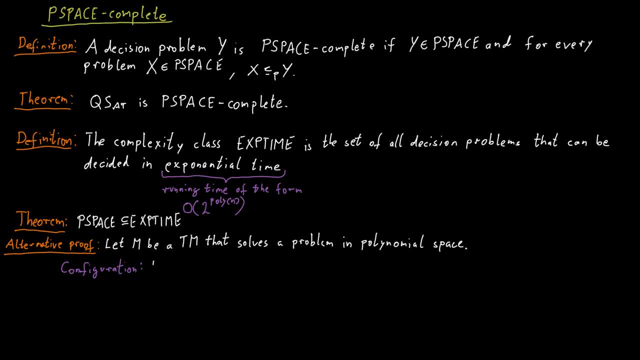 and its current situation completely So. it describes where exactly the head of the Turing machine is on the tape, It describes the entire contents of the tape And it describes the internal state of the machine as well. A Turing machine that only uses polynomial space. 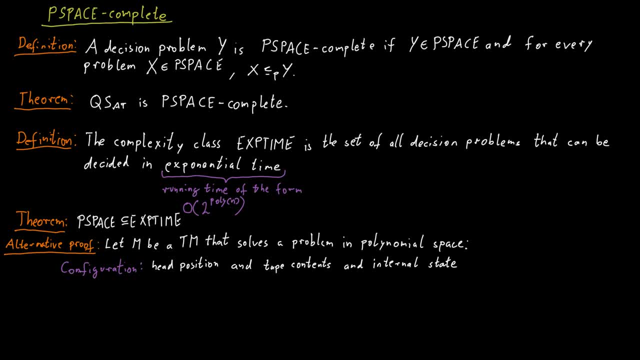 can only have an exponential number of different configurations. The reason is that if we only use polynomial space, really only a polynomial number of cells of the tape are important, So we only need to worry about what is stored in those cells, because we will not be able to modify anything outside of those cells. 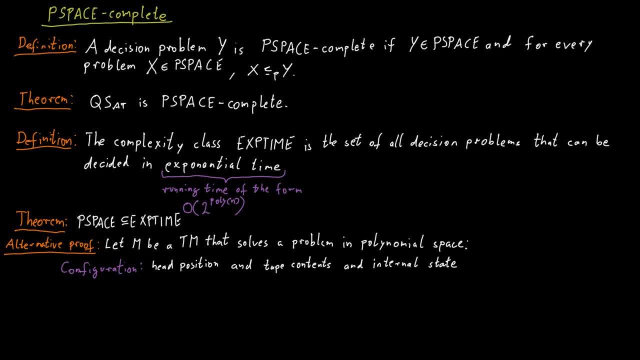 And also the head of the Turing machine must point to one of those polynomially many cells. So what are the different contents those cells can have? So each cell has a symbol from the alphabet written on it, And so let's say we use space p of n. 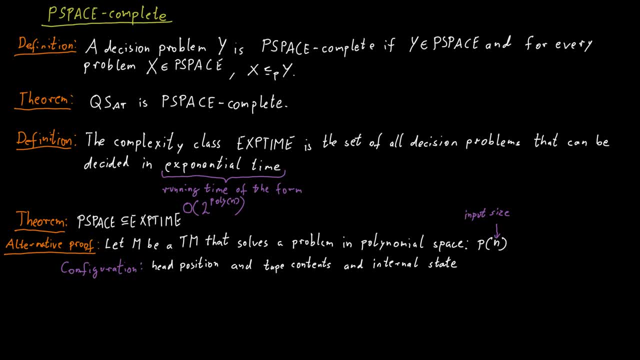 where n is the size of the input and p is some polynomial function, Then in each of those p of n cells that we care about, there can be a symbol from the alphabet, And that gives us, in total, a possible combination of contents for the tape. 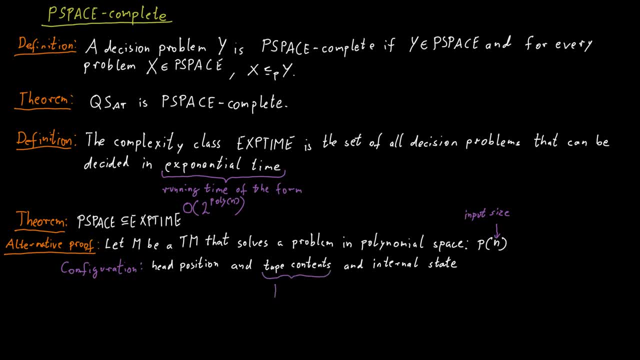 that is equal to the size of the alphabet, to the power of p of n. In addition to this, the head of the Turing machine can point to any of these cells. So the number of configuration is multiplied by the number of possibilities of head positions. 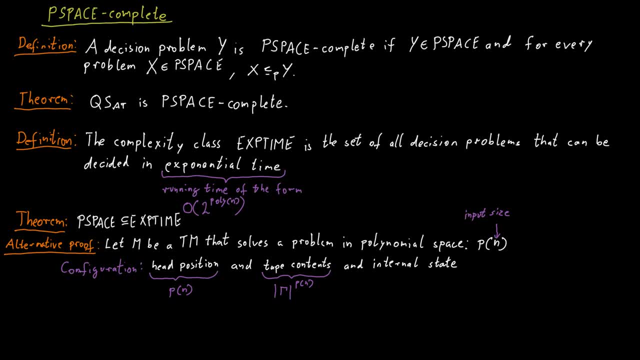 So we need to multiply this by p of n, And then also the Turing machine can be in any of size of q, many internal states. So we have to multiply all of what we had before times that, because those are the number of possibilities for the internal state. 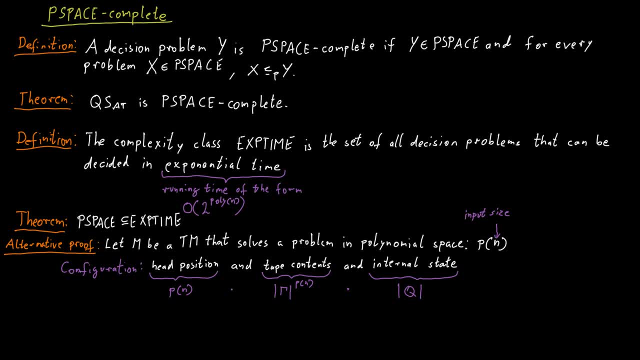 times the number of possibilities for the head position. times of the number of possibilities for the contents of the tape. So those are the total number of configurations. Size of the alphabet to the power of p of n times p of n times the size of q. 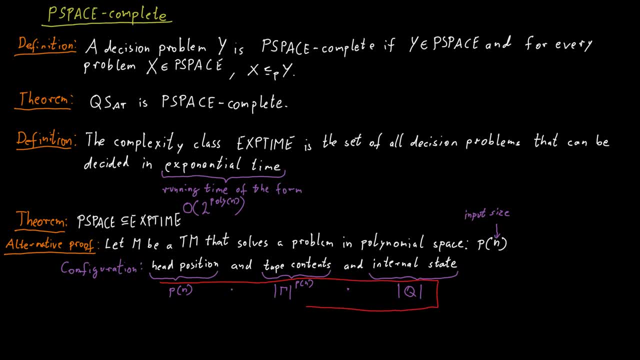 So we can only have an exponential number of different configurations of this polynomial space Turing machine. Consider what happens if, during a computation of the Turing machine, we encounter the same configuration twice. So we encounter the configuration, we continue our computation and then, at a later point, we encounter the same configuration again. 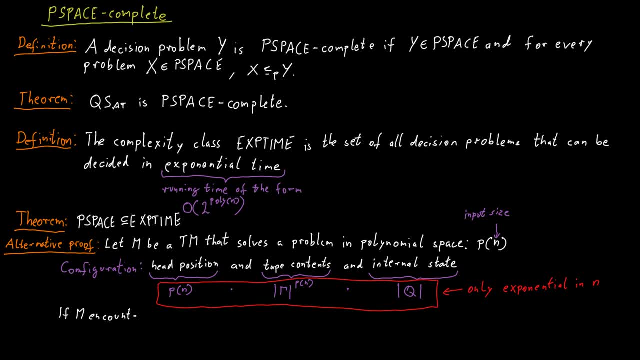 What will happen in this case? In this case, the Turing machine will enter an infinite loop, So it will go through that configuration again and again and again. It will follow the same kind of computational actions it took between the first time it encountered that configuration. 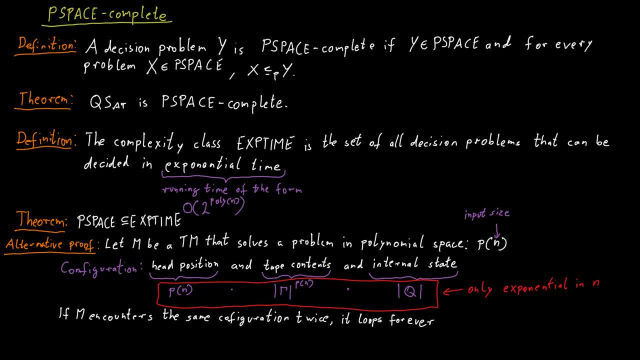 and the second time it encountered that configuration And it will go through this process again and again and again. Therefore, the Turing machine will not terminate. And we said: a Turing machine that doesn't terminate doesn't compute anything. And because of this, if we have a polynomial space Turing machine, 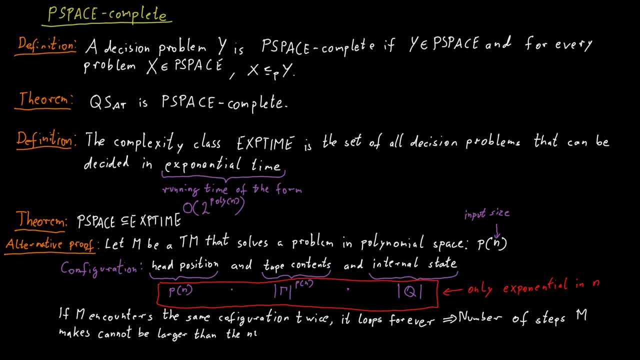 that does compute something. it can only take exponential time. If it would take more time, it would, by the pigeonhole principle, encounter the same configuration twice and enter an infinite loop. To summarize, we know that p is contained in Np. 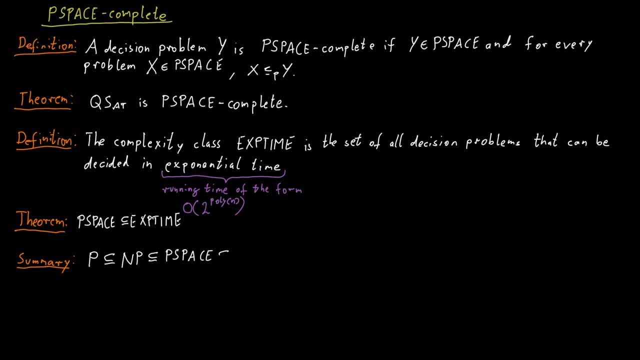 and Np is contained in p-space and p-space is contained in exp-time. As we've emphasized many times, we do not know whether p is equal to Np or not. Also, we do not know whether Np is equal to p-space. 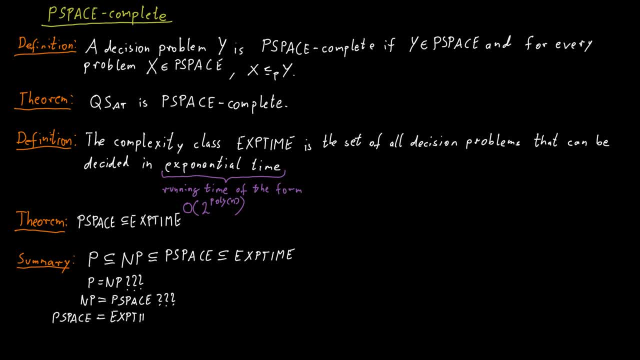 And we also do not know whether p-space is equal to exp-time, So it could be that any of those subset inclusions here are actually equalities. However, what we do know is that p is not equal to exp-time, So there are really problems. 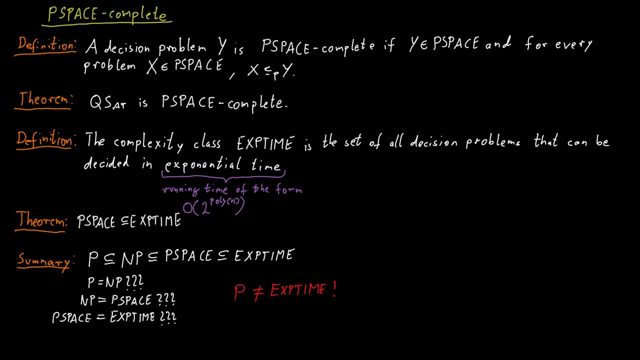 that can be solved in exponential time, which we can prove cannot be solved in polynomial time. So the first set in this series of inclusions is not equal to the last set And therefore we know that one at least one of these three inclusions. 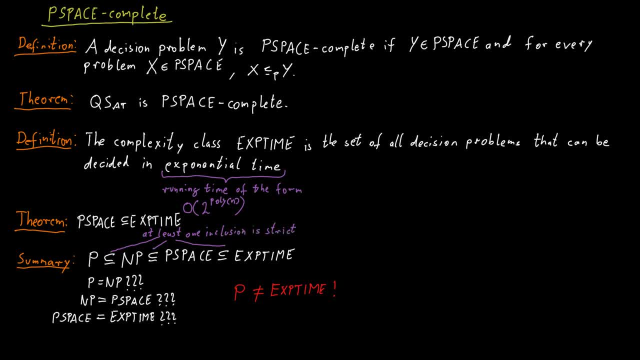 is strict, But we do not know which one. Most people conjecture that all three of them are strict, But, as I said before, this is not clear. We don't know for sure.